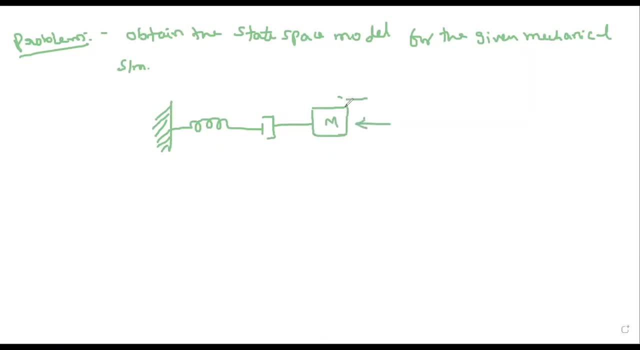 And force is applied to this. Therefore displacement will be in this direction. only Say: force is F of t And the displacement is Y of t. Here the dash rod discuss: friction Proficient is B and the spring constant is K. 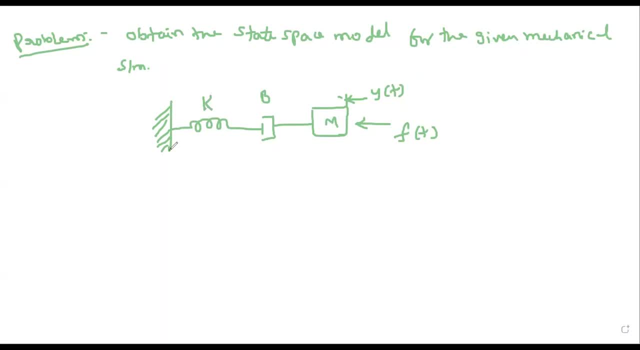 And here there is no. there is no friction between this. We have zero friction here. Alright Again, This is the given mechanical system. For this we need to obtain the state space representation. So we will see the solution. 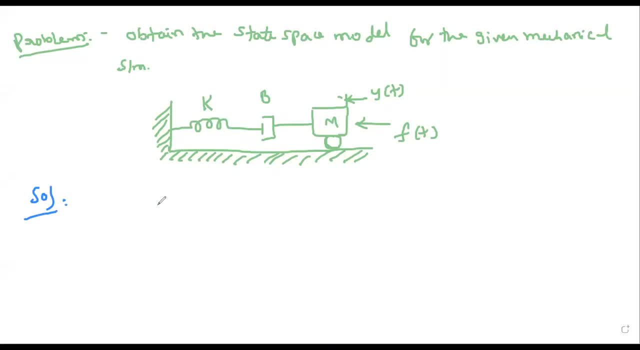 For getting this state space model of a given system. we need to write the differential equation here from this. so mathematical relations here, kvl, kcl, we can't do right. we can write only the force balance equation. what is that? applied forces? sum of applied forces is equal to sum of the opposing forces. 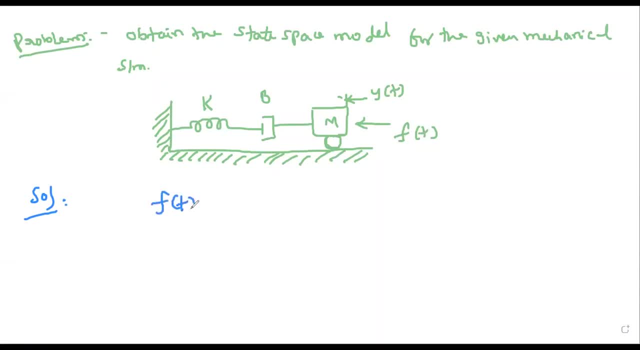 here the applied forces f of t, only one force that is equal to the opposing forces. sir, how many opposing forces are there? three? what are those? mass, sir? what is this? b, sir? b is the viscous friction coefficient dash part. this dash bar viscous coefficient is b, b and yeah, this is b. 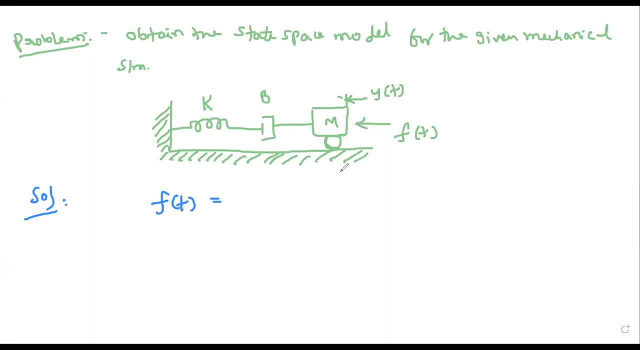 and this is k spring constant. now tell me what is the f of t formula? the opposing force due to the mass, plus opposing force due to the dashboard spring. what is fm force acting on a mass body? f is equal to, f is equal to ma. force acting on a mass body, m into a, so mass into acceleration, the acceleration in terms. 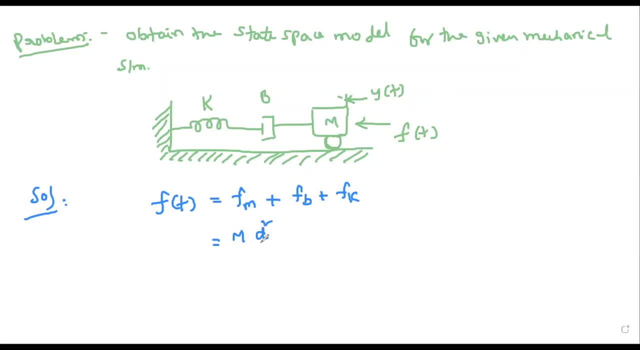 of displacement. we should write: that is b square by dt, square of y of t, plus opposing force acting on dashboard. remember that's it. this is the force equation. from this differential equation we should write: we should represent in the state space model. here we need to select state variables to represent a model in the. 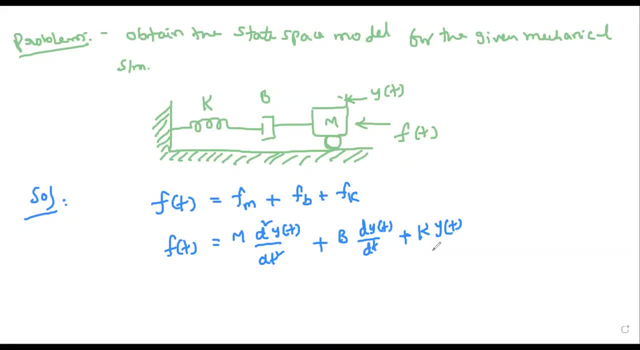 state space, its representation. we should find out what are the state variables of the system in this kind of, in this kind of system. there is no storage element here. I mean, we can't define exactly what is the storage element here, there, for this not electrical system. we don't know what is there in the mechanical. 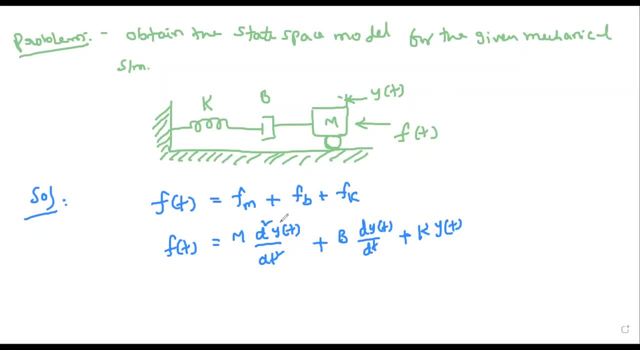 system. so if you have a differential equation, there is a different processor. I'll tell you. first of all, we should understand how many state variables we should select. how many we should select the degree of the derivatives: highest degree. since it is a second order differential equation, we should take two. 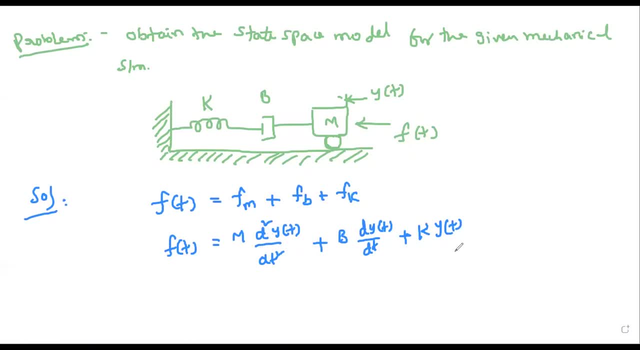 state variables from this. okay, in that first one is last y of t, we should select this is the first state variable and next d Y by D T should be selected as d T x2 state variable. whatever the differential equation processor is same. first y of t. whatever the output variable, you take it. 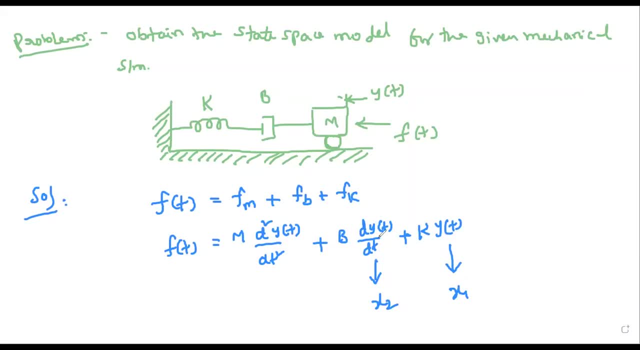 as there X one state of variable and it's derivative for start, derivative as the X two variable. If you have a third order differential equation, then next to X three, we should select this B square, Y by DT square. Okay, Since it is a second order differential equation, we need to select only two. 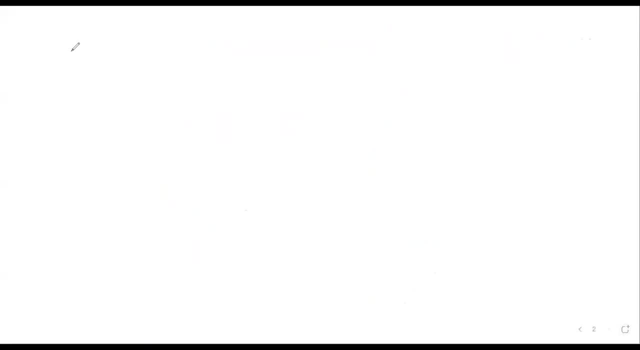 So that we selected already. then leave it. Now we'll write: what is the state, variable state where it was X one is equal to Y one and X two is equal to D by one. sorry, D Y by DT. It is not Y one, it is Y one. 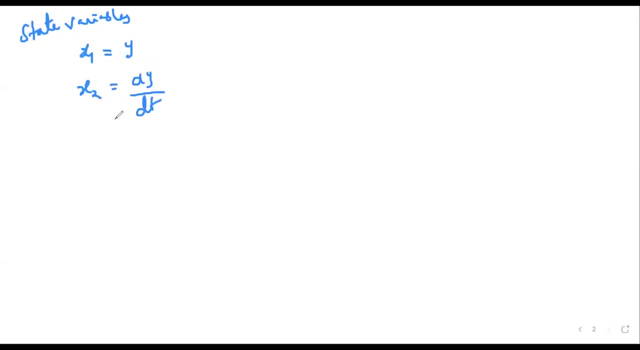 So we have Two variables, now state variables. that is done. Now what to do next? differentiate X one dot, X two, X one dot. we should find what is X one dot, D Y by D T, D Y by D T. That is equal to X two, X two. next, X two dot. we should find D square, Y by D T square. 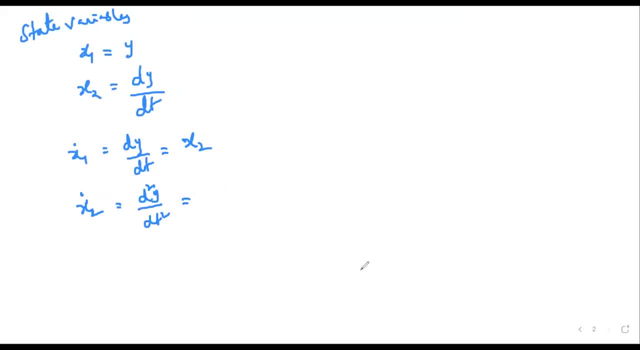 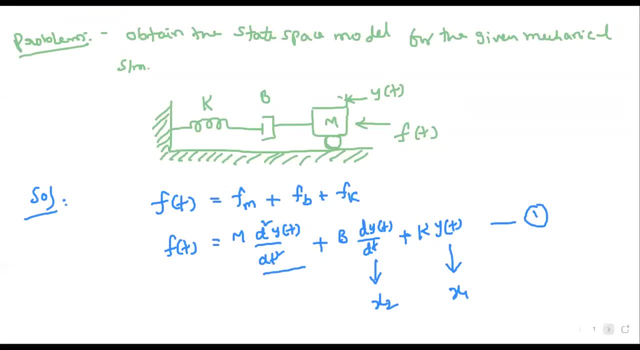 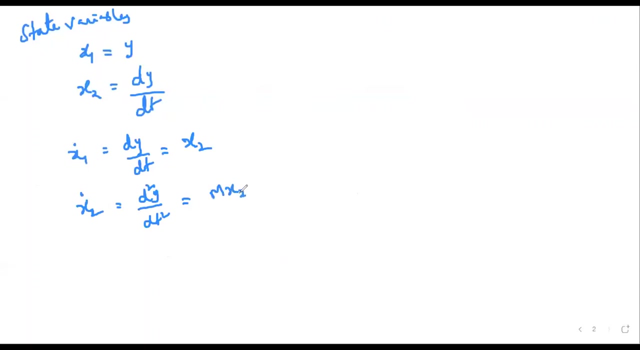 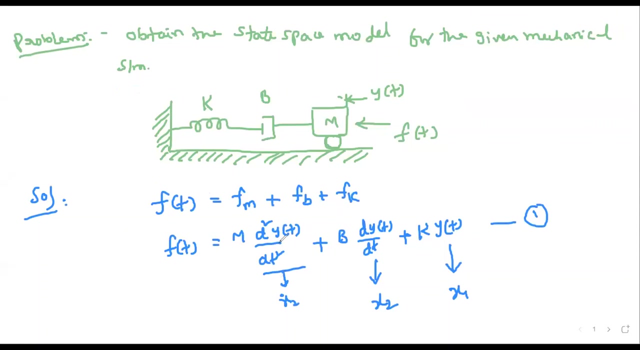 Very good. What is this? Nothing equation. we can get this Right. Yes, sir, Tell me The next two dot: X two dot. No, no, no, no. This is X two dot. I should derive it. This is equal to. 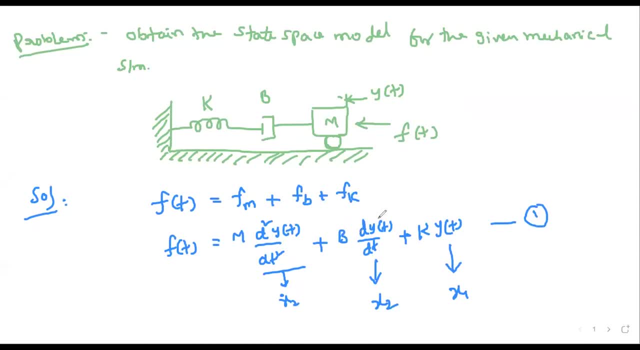 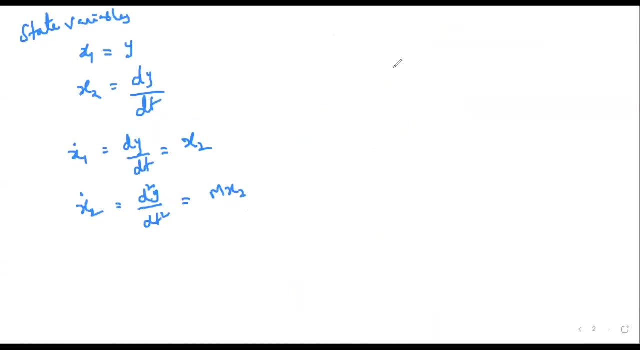 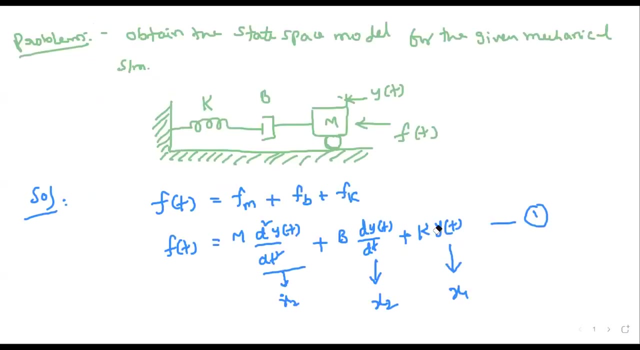 That means F of D, minus this We should have Okay. Minus this divided by M, Correct, Yes. So that way you should tell First what is the X1 factor Here. this is X1.. So minus K by M it will come. 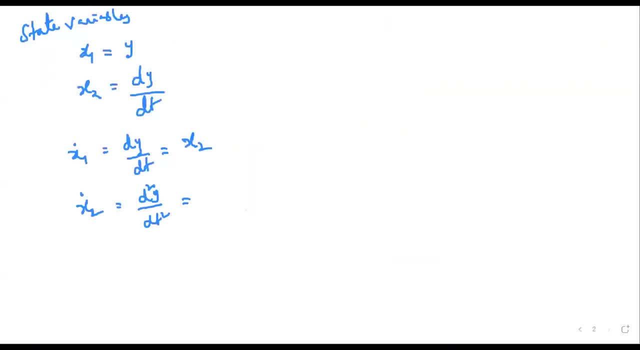 Right, I will write here Better From the first equation. what I can write is: M into D square, Y by DT square is equal to F of T minus B into D, Y by DT minus K into Y. Here this is nothing but X2 dot. 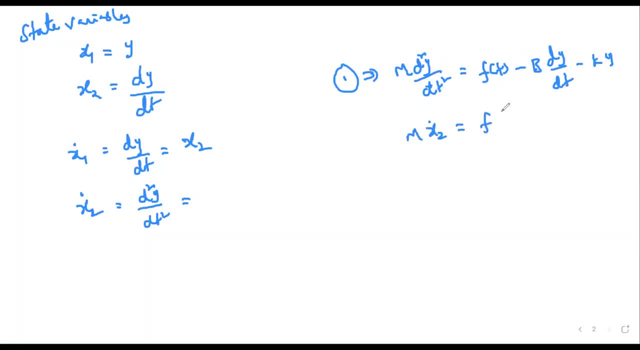 M. X2 dot is equal to F. Here I will write F only Minus B into this: is X2 minus K into X, So X1.. Therefore X2 dot- how to write It- is 1 by M into F minus B by M. 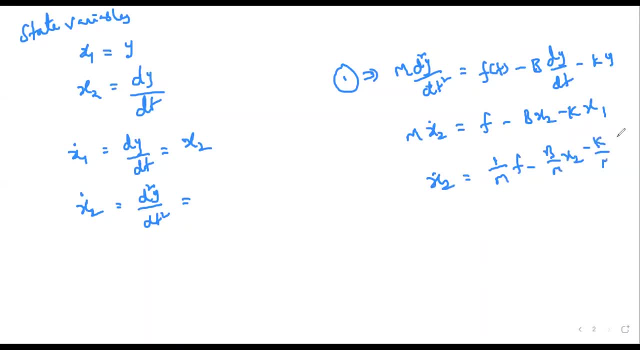 into X2, minus K by M into X1.. From this I will write in the order. Therefore, it is minus K by M into X1, minus B by M into X2, plus 1 by M into F. Okay, Yes, sir. 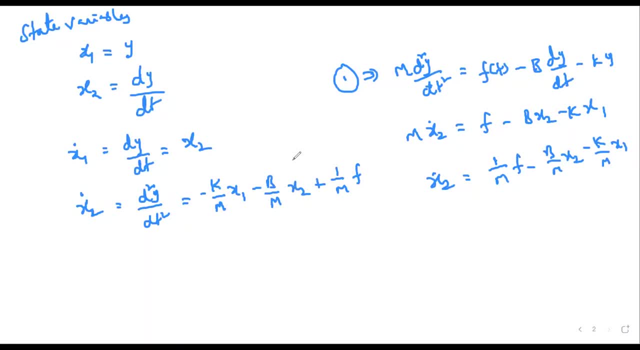 Now this F is nothing but U. Right, I cannot equal to U, So I will write here itself: This is U Input. Input is the force, So here I can write U. Therefore we have equation 2 and equation 3.. 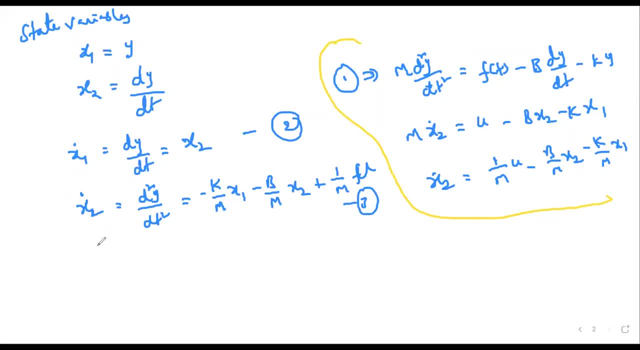 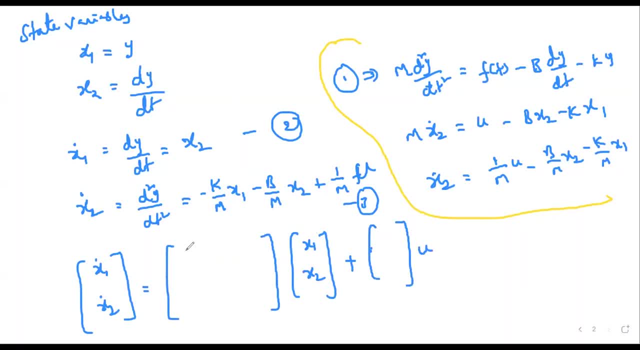 u then tell me what is this: 0. this value 0. 0. next value: 1. 1. next minus k by m. minus k by m. next minus b by m. very good, next u: 0, 0, 1 by m. very good, that's it. so we got the state equation now. 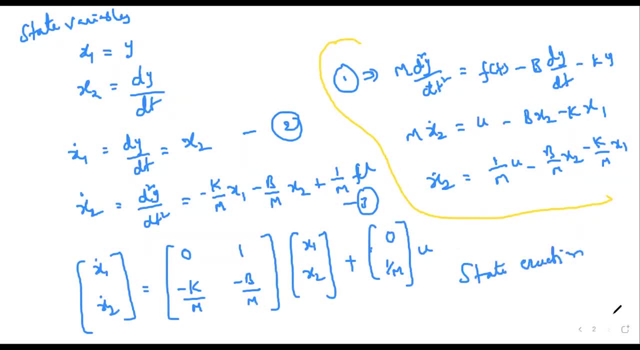 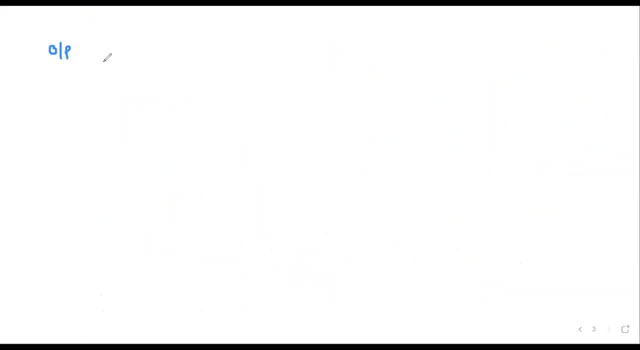 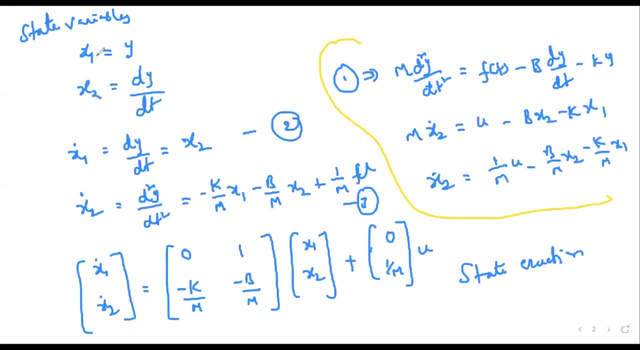 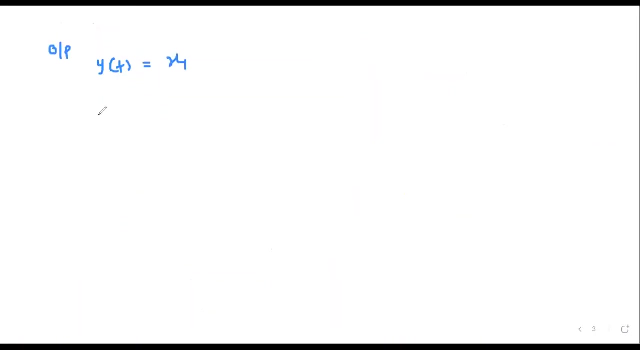 done. next we will see the output equation. how to get the output equation. output is y character displacement, so output y of t is equal to, in terms of state variables and inputs. what is y of t is equal to x1. right, since x1. y is equal to x1. x1, 1, 0, x1 into x1 into x2 is equal to matrix. 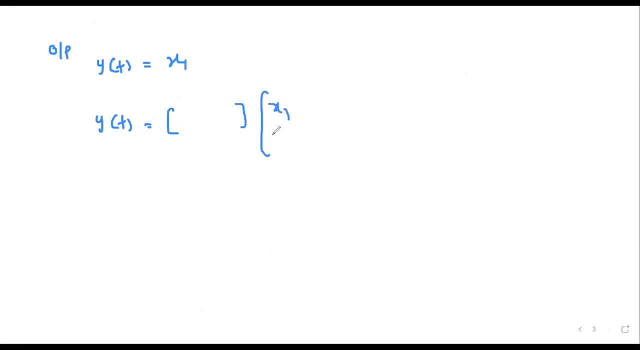 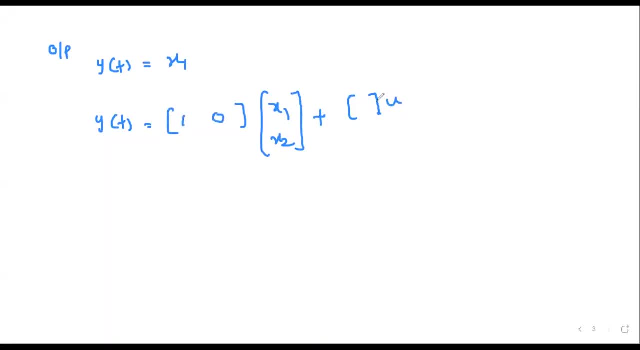 1, 0.. 0, right, Yes, 0.. This is the output equation. That's it Over. Therefore, state space representation is x, dot is equal to ax plus du and y is equal to output. y is equal to. 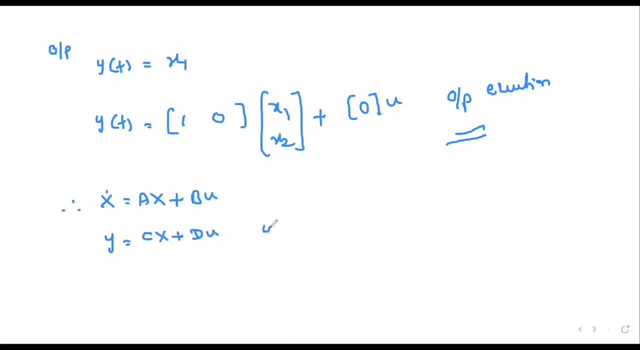 cx plus du, where a is equal to 1, 0 minus k by m, k by m minus b, by m minus and b is equal to 0 minus 1 by m plus 1 by m c is equal to 1, 0.